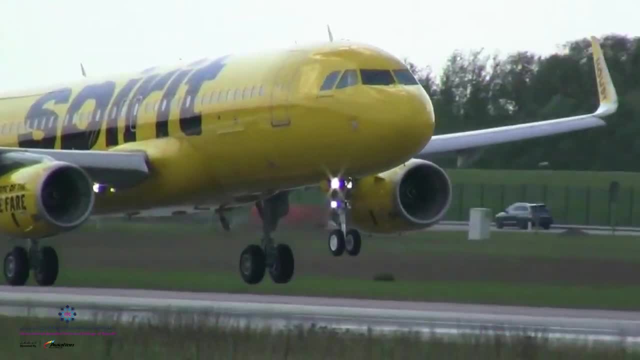 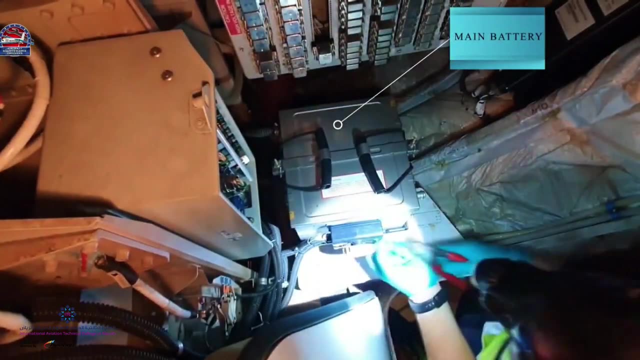 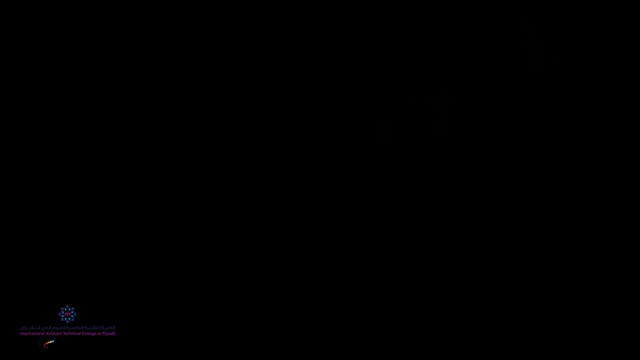 the ram air turbine, An emergency electrical and hydraulic backup located in the belly, fairing down to the batteries. all form part of the aircraft electrical system for a typical large aircraft, in exactly that order from top down. in case of failure of each Turbofan engine, generators provide electricity through the AC bus In order to ensure constant. 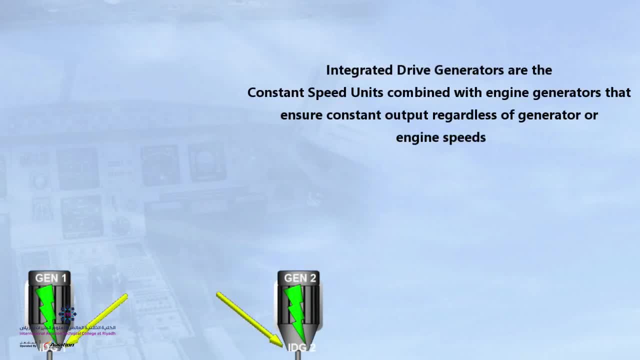 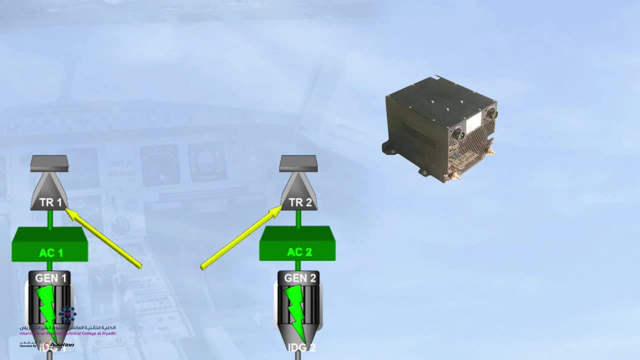 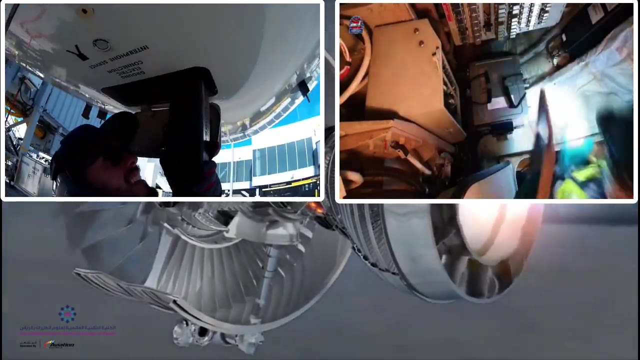 output generators on a complex jet aircraft are connected to the integrated drive generators on each engine. A transformer rectifier in the system will convert so produced AC to DC and route it to where it is needed through the DC bus. The entire system is backed up, however power. 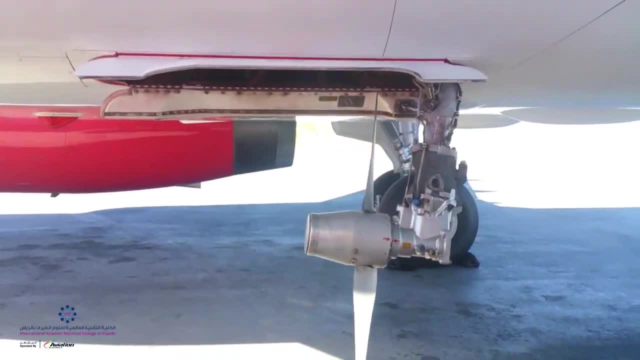 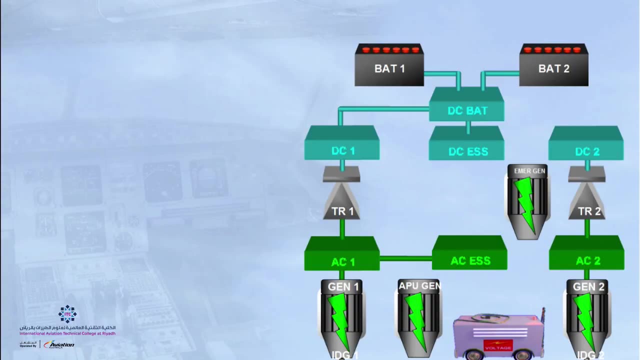 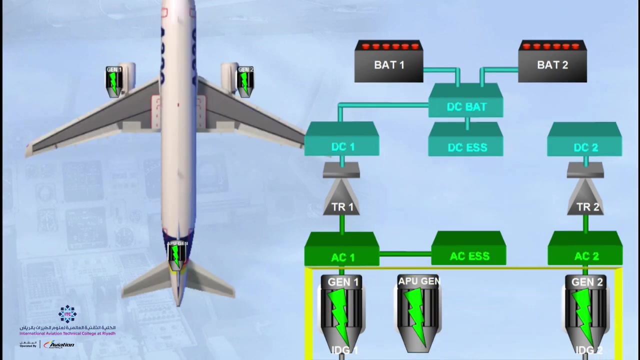 sourced from the backup systems progressively degrade, like from the ram, air turbine or the batteries, and will route to essential systems critical to safe flight only after going through either of the rectifier or inverter stage. Either of the auxiliary power unit or the two engines can support the DC bus. Either of the auxiliary power unit or the two engines can support the DC bus only after going through either of the rectifier or inverter stage. 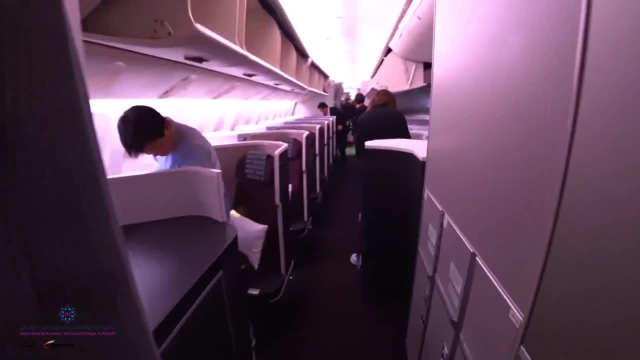 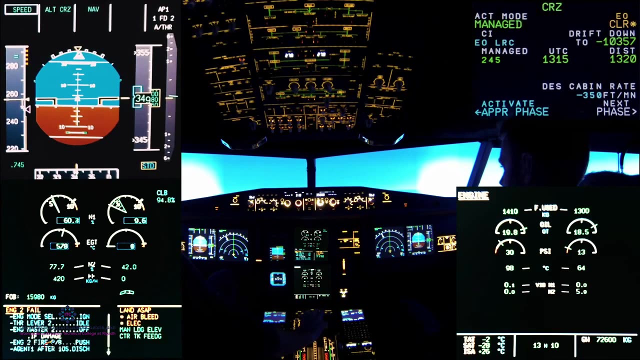 The power system will then use the power supply of the entire aircraft. In event, it comes to the battery stage for the final backup, after every other source of generation has gone belly up, since they produce direct current. an inverter will convert the direct current. 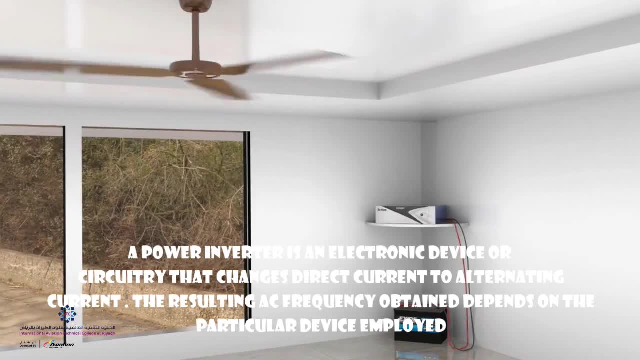 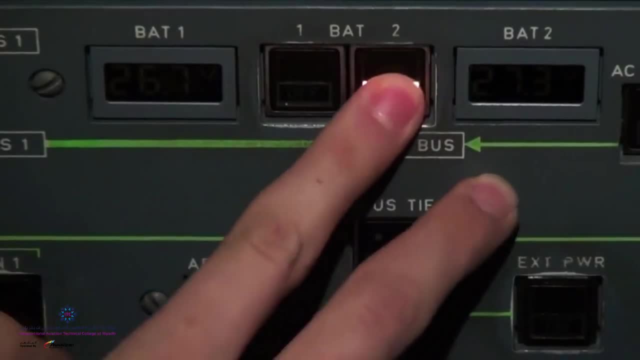 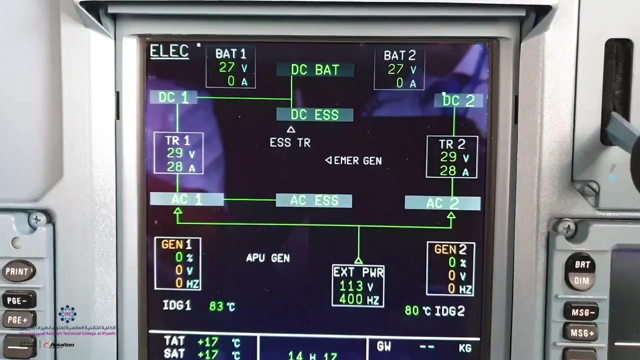 coming from the batteries, allowing systems to power up on alternating. current Battery is the last source of electric power on the aircraft, so ensuring that they have enough juice before engine start is a normal checklist item, also to monitor that enough charge being maintained on the battery during flight. in a typical automated system, batteries on both sides. 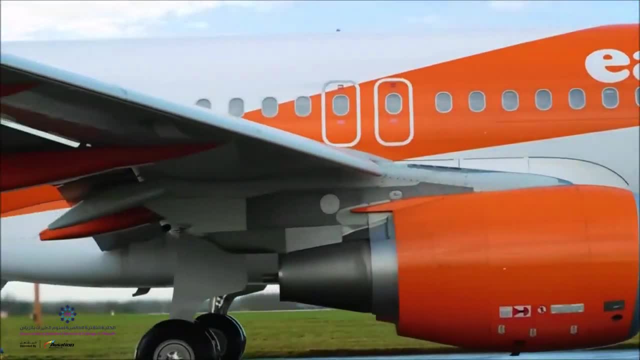 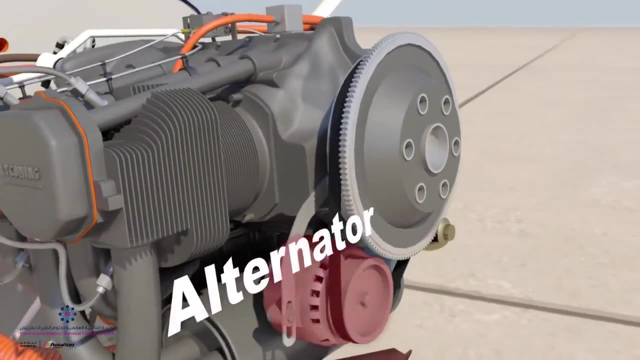 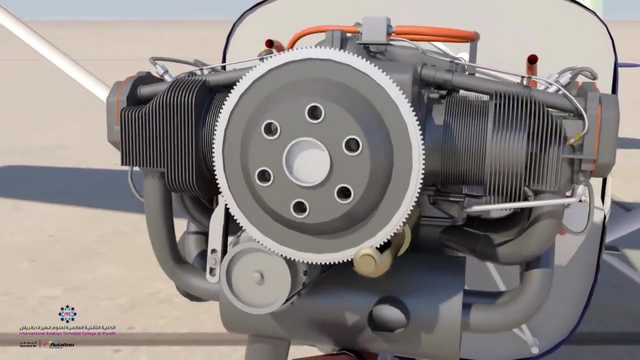 will charge through the dc bus when main engines are running. a smaller airplane would either have a generator or an alternator. both provide dc power. for example, on a cessna 172, electric power is routed through a dc bus that aids engine starts, lights, movement of flaps, instruments. 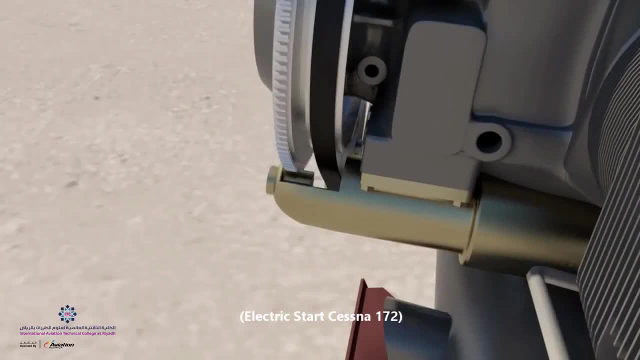 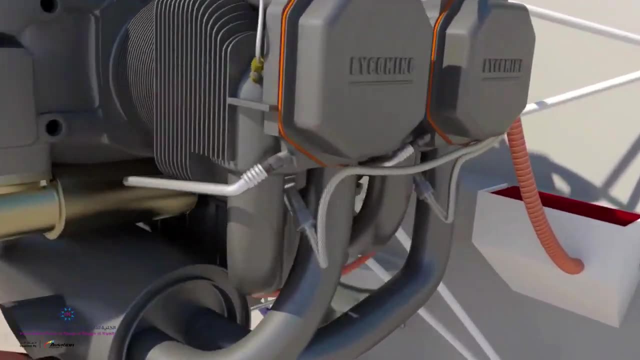 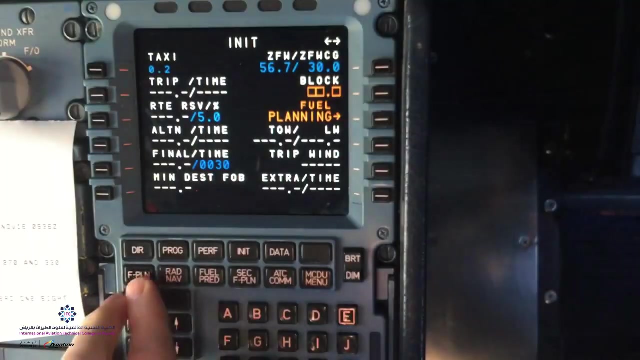 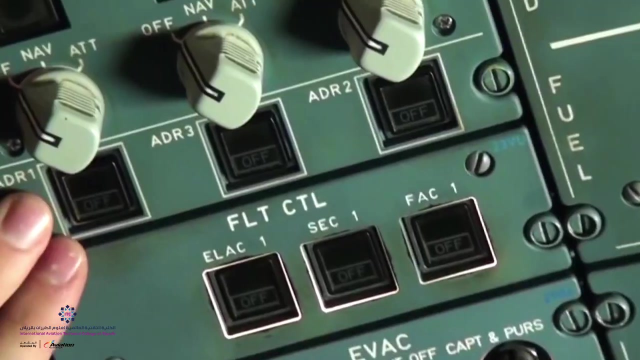 nav aids and radios. on engine start battery becomes part of the electrical load while being charged by the generation system on it too. battery is the last chance power backup on the larger, more complex aircraft electrical system. power is supplied to flight management computers, displays, lights, flight instruments, radar and other avionics. in addition, you would have the 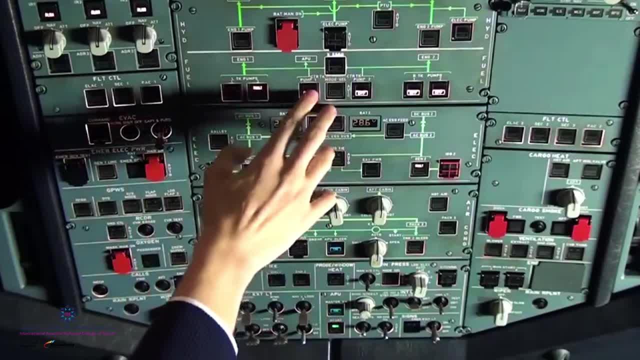 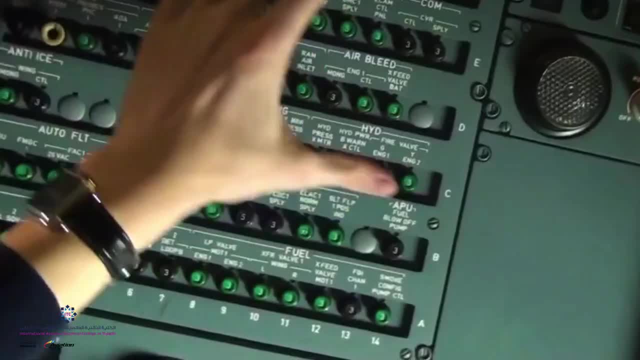 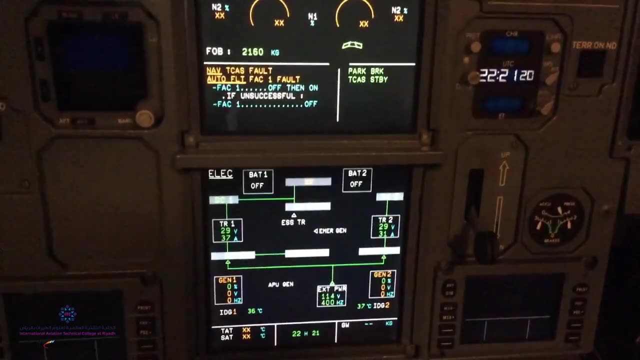 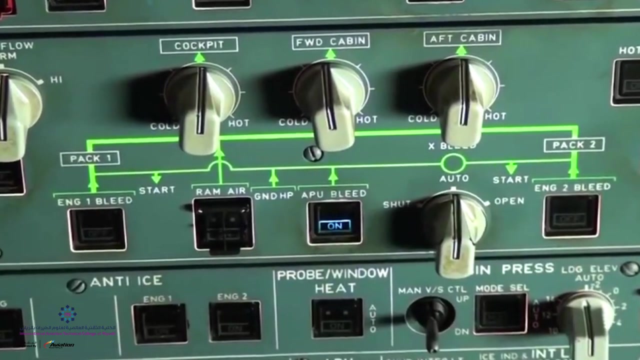 navigation, communication, fuel and hydraulic pumps and so on, breathing on electricity produced by the engine generators. these systems are protected by various types of circuit breakers from inadvertent surge in electric load. failures are indicated in the cockpit as a caution or warning to which pilots take appropriate action. per the aircraft sop from the cockpit, a whole panel would be given for. 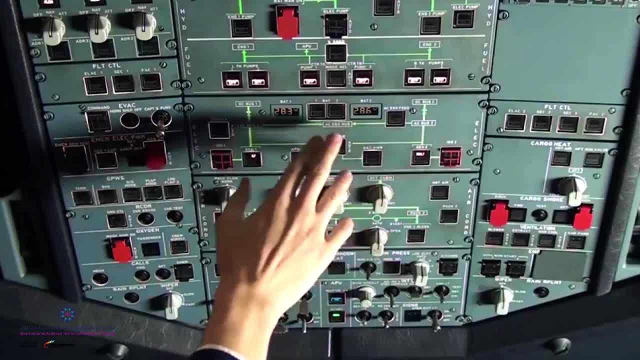 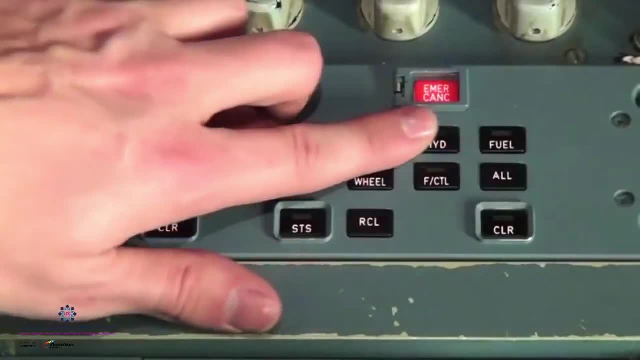 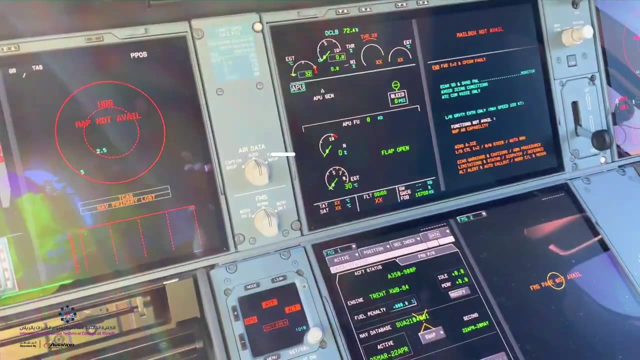 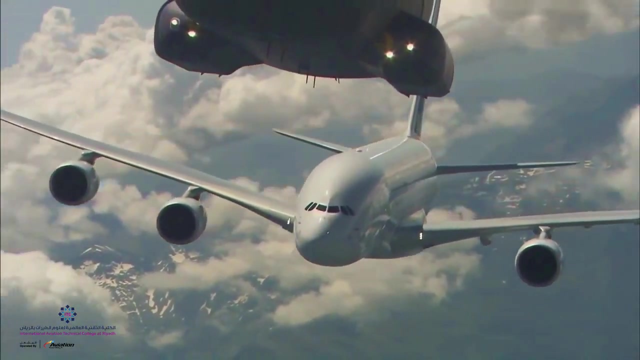 managing aircraft electrical system. indications would appear on corresponding displays. modern electrical systems have a separate electric panel for managing emergency systems from displays. you could monitor battery and rectifier status, apu generators, external systems and emergency management, etc. each plane comes with its own distinct system, but at least all of them work. 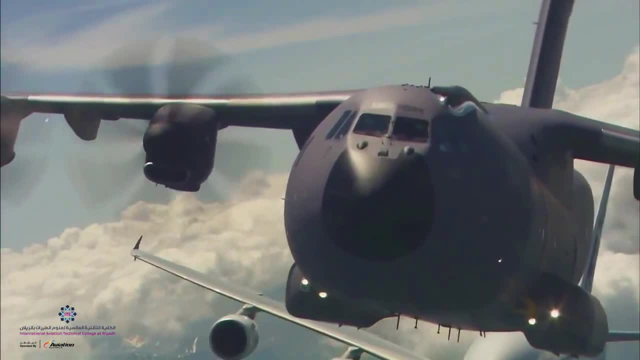 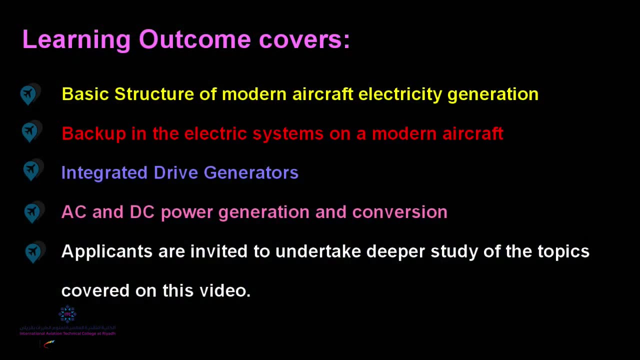 in the basic fashion and unless, of course, contemporary systems give more weight to solar alternates, more or less we'll be living with the ground level schematics for a while. have fun, you. 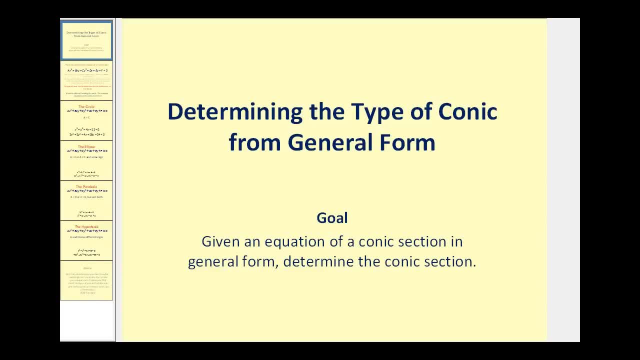 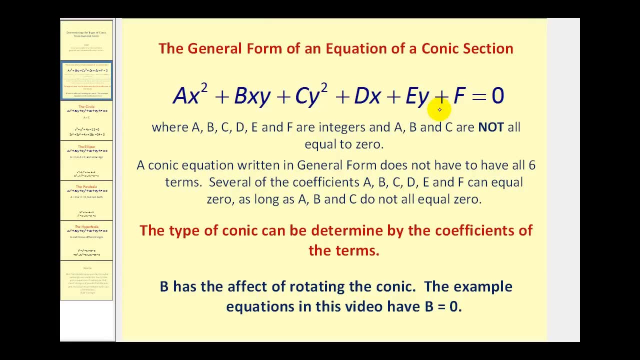 Welcome to a video on determining the type of conic from the general form of the equation. Here we see the general form of an equation of a conic section where a, b, c, d, e and f are integers and a, b and c are not all equal to zero. Notice, if a, b and c were. 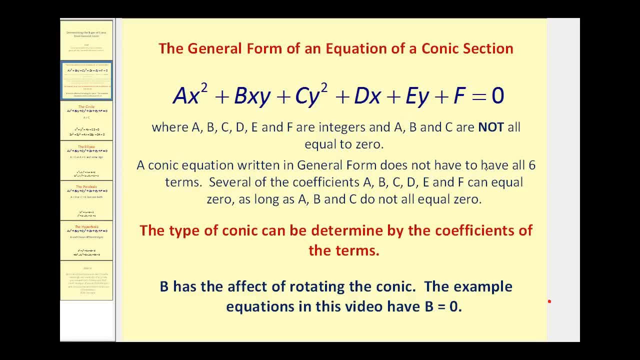 equal to zero, we'd have a linear equation. A conic section, written in general form, does not have to have all six terms. Several of the coefficients can equal zero as long as a, b and c are not all equal to zero And the type of conic can be determined by the